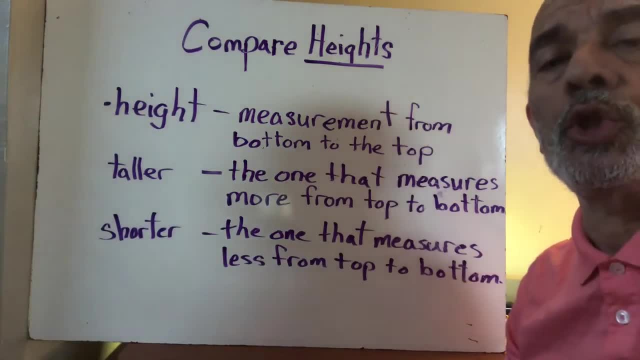 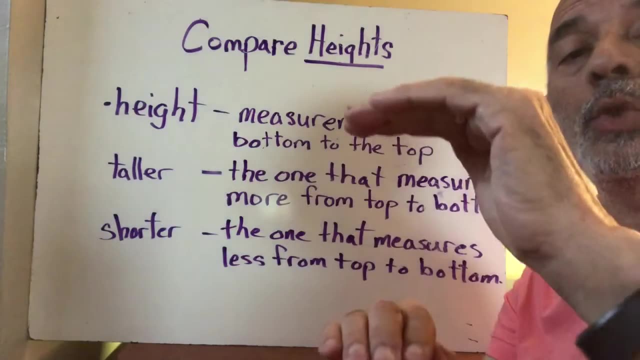 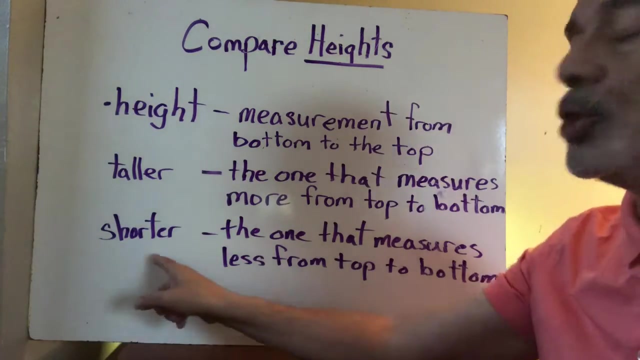 from the bottom to the top. that one is called the taller one. That one is the taller. The shorter one is the opposite. If you're comparing two objects and one is shorter than the other one, then that one is the shorter one. 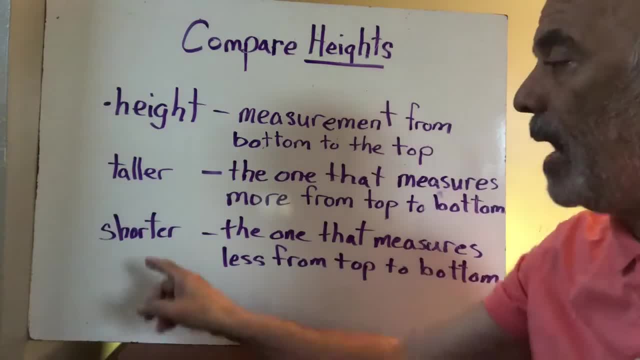 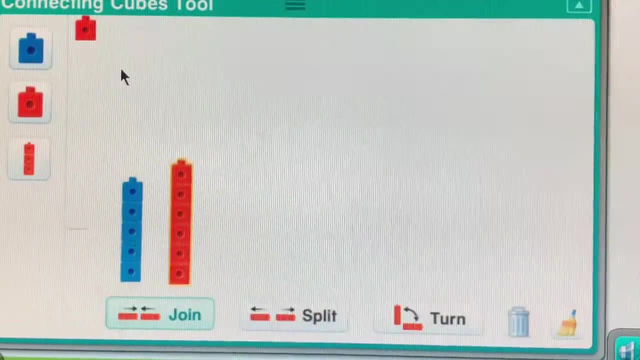 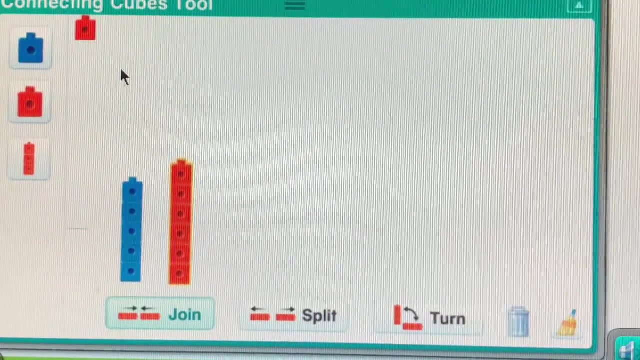 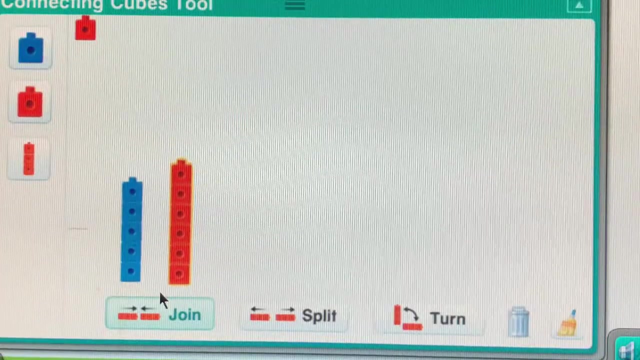 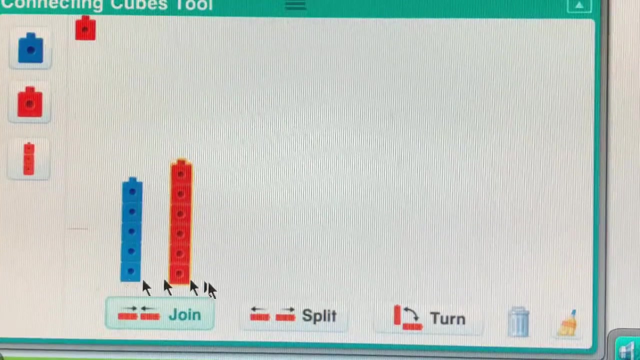 If one is lower than the other one, that one is called the shorter one. How can we compare the height of two objects? Which of the cube towers is taller? To compare the height of two objects, it should always be lined up evenly at the starting point. 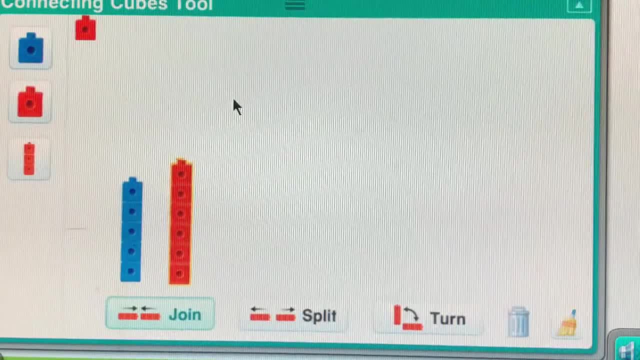 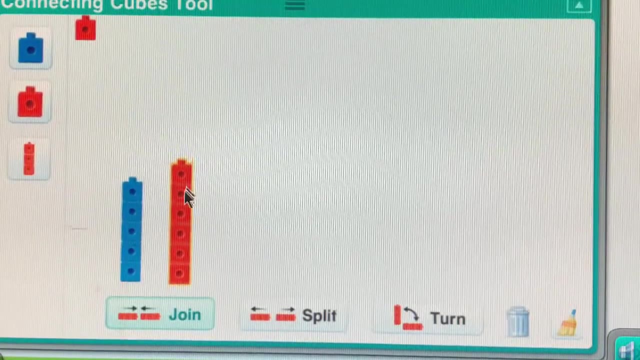 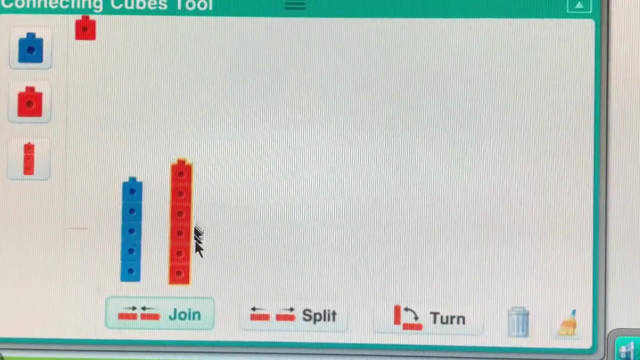 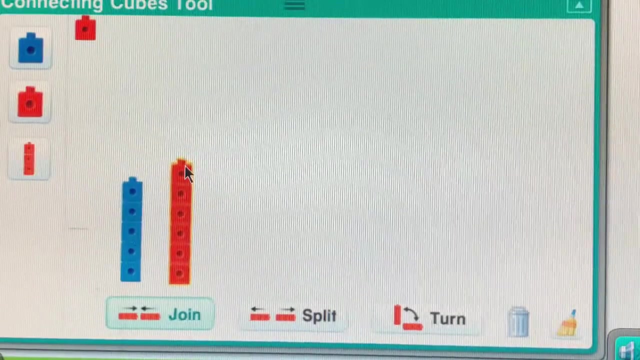 The tower that goes up higher is the taller one. Let's look at these two towers. Which one is taller? Well, we can see this one is. So the red tower is higher. That means that the red tower is taller. The blue tower is shorter. 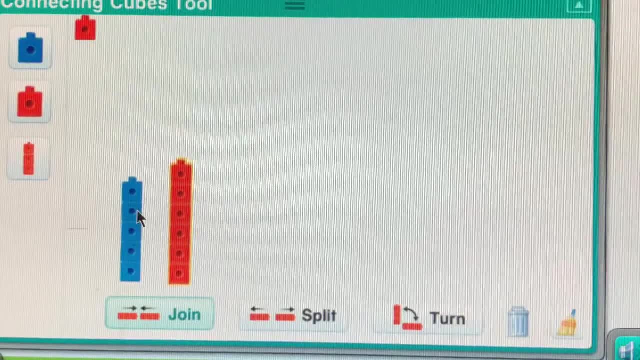 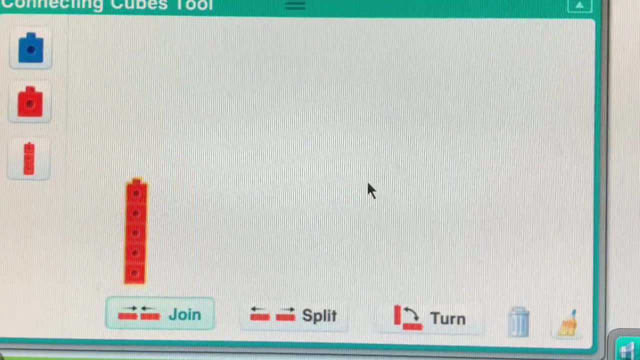 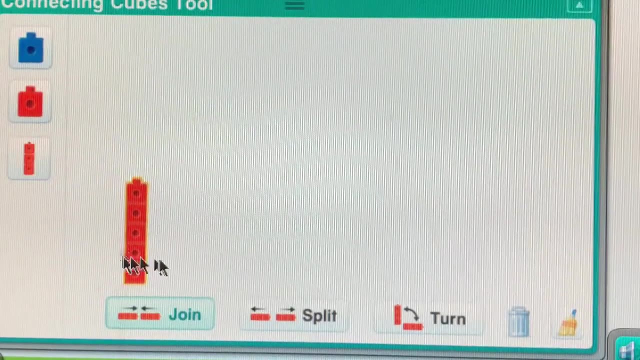 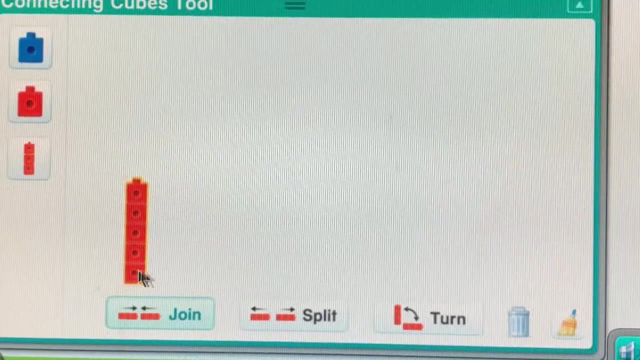 It doesn't go up as high, so it is shorter. Let's make a tower that is taller than the red tower. We can do this by counting how many cubes- 1,, 2,, 3,, 4, 5- are in the red tower. 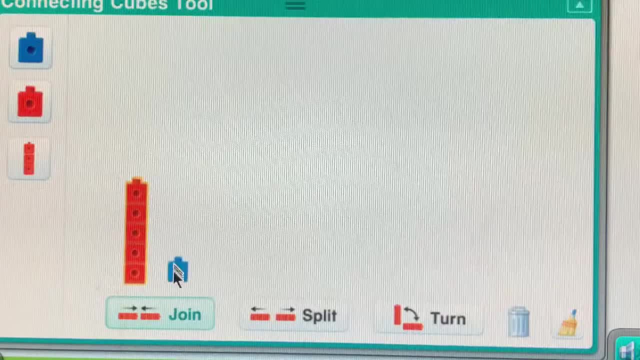 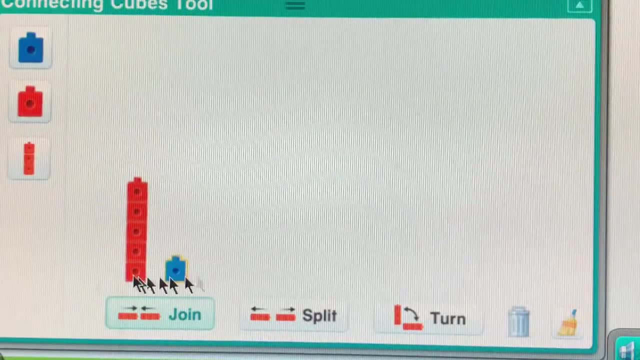 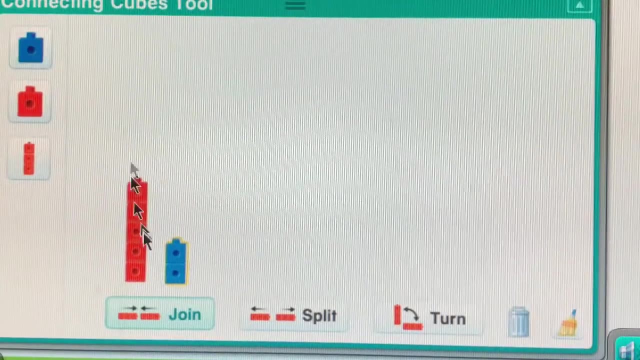 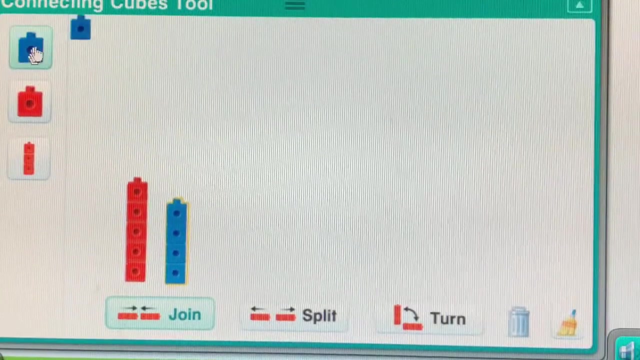 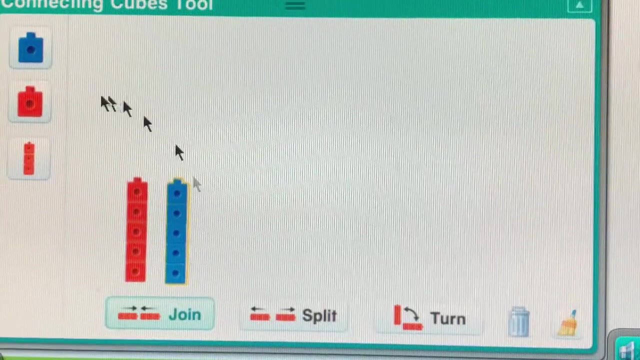 And then we will build a tower that is taller by adding cubes, Start at the same place, Then we will add some cubes until the tower is taller. They both have five cubes, so now they are the same height. If I want to build a tower that is taller,